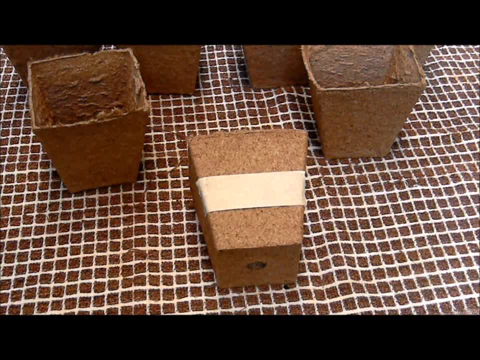 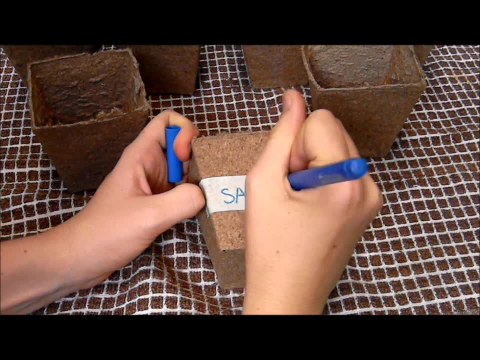 off enough to fit across the length of the pop plant. Using a text or a pen, write the type of soil that is going to be poured into the pop plant. Repeat this step to all. eight pots have been written on Step 2. Place gardening gloves on hand place. 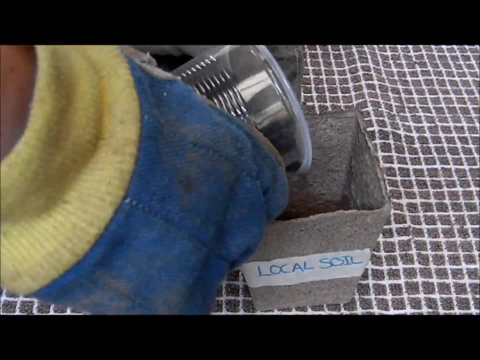 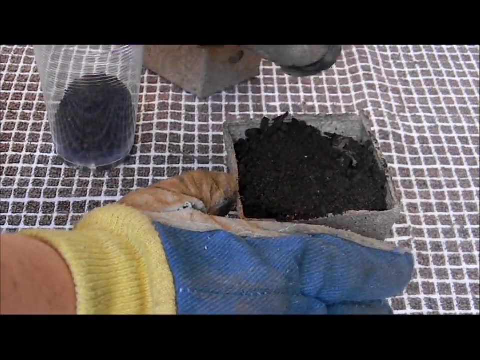 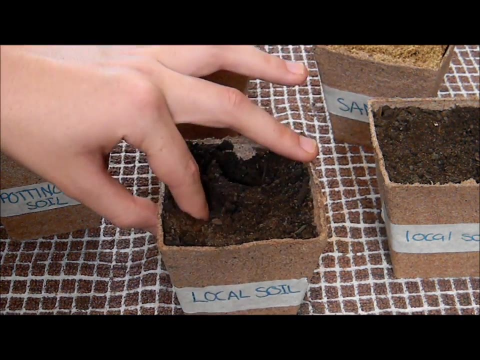 your hands and then grab the first pop plant and place upright on the table. Pour the soil into the pop plant till the soil reaches the top, Then flatten with your hand and repeat till every pop plant is full with each soil. Step 3. Using a finger, make three small holes. 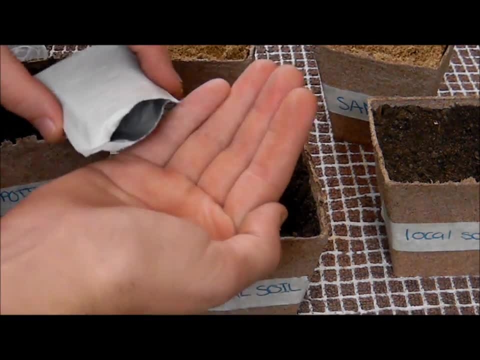 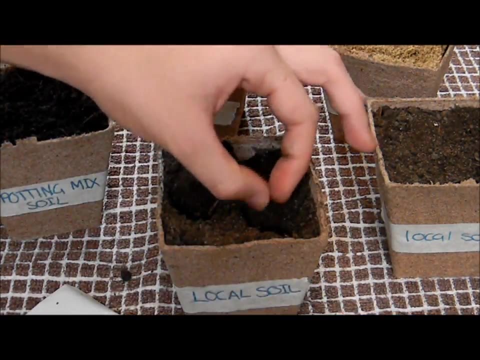 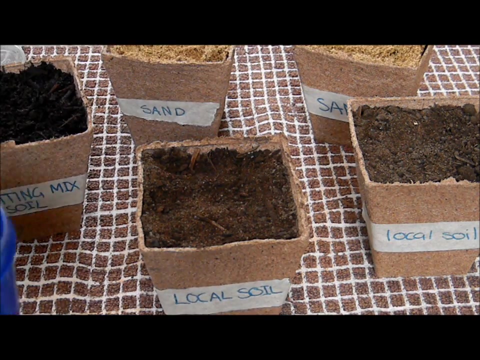 a couple millimetres deep and apart from one another. Open the packet of seeds and pour a few in your hand. Place a couple of the seeds in each hole and cover up the holes with the dirt using your hand. Step 4. Using half a cup of room temperature water, pour over the pop plant. allow the. 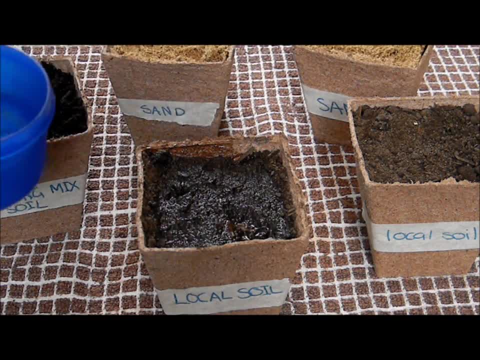 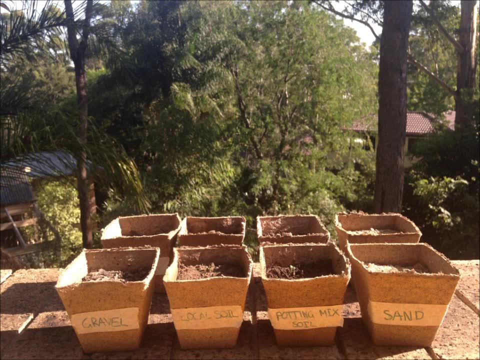 water to soak in first and pour over the rest in small amounts. Repeat this for all pop plants till all of them are watered. Step 5. Once all eight pop plants are watered, place outside where the plants have had enough sun for days. Every second day, water all. eight pop plants. Make the first observation of the pot plant. Place the pot plant on the ground and then place the pot plant on the ground. Repeat this step for all pot plants. Step 5.. Once all eight pop plants are watered, place outside where the plants have had enough. 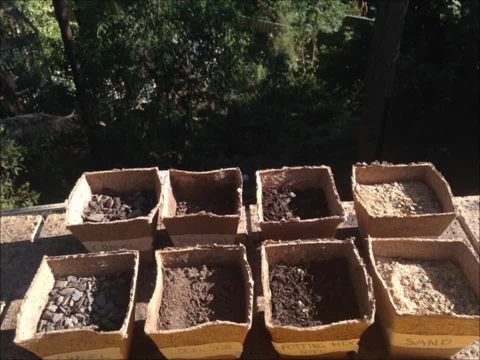 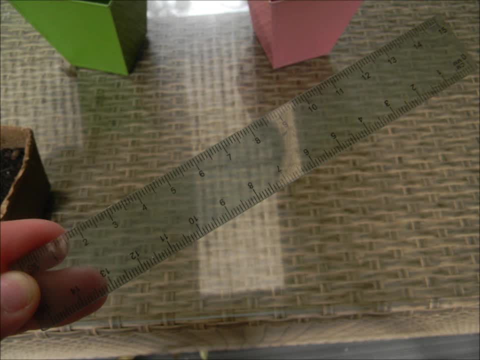 sun for five days and then place the pot plant on the ground. Repeat this for all pot plants. Take photographs of each observation and measure the height of each plant, Measuring the plants. After the first week you will notice the plants have started to grow By using a ruler. measure the height of each plant by placing